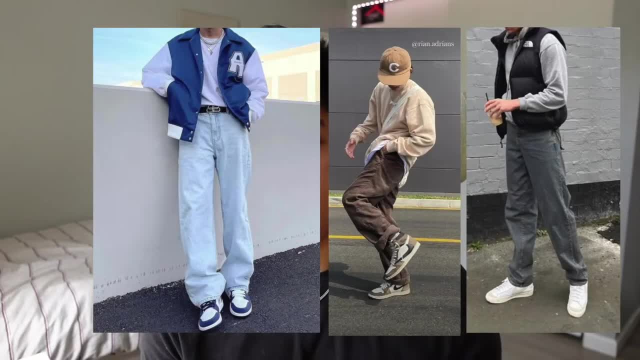 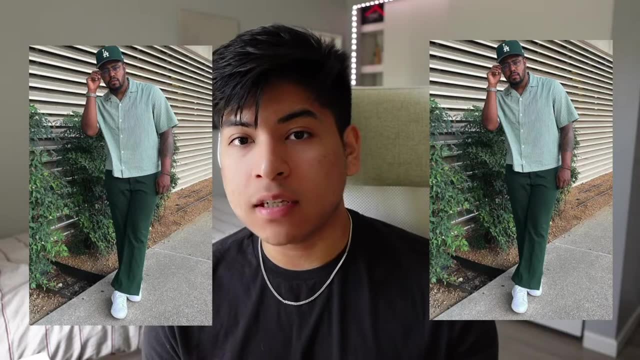 different types of shades, tints and saturation pieces into your outfits, Like this one, for example. the primary color on this one is green, but the top piece has a different type of shade or tint variation of the color green, which gives it a layer of color and more depth to it. 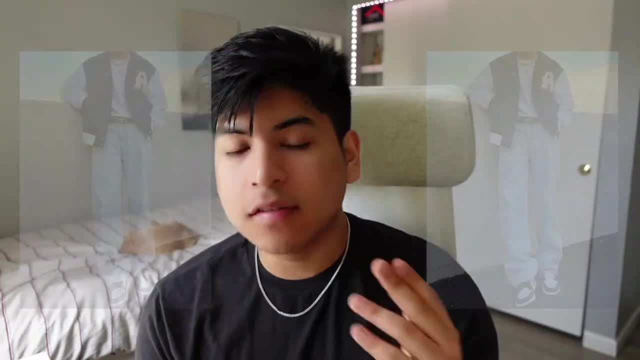 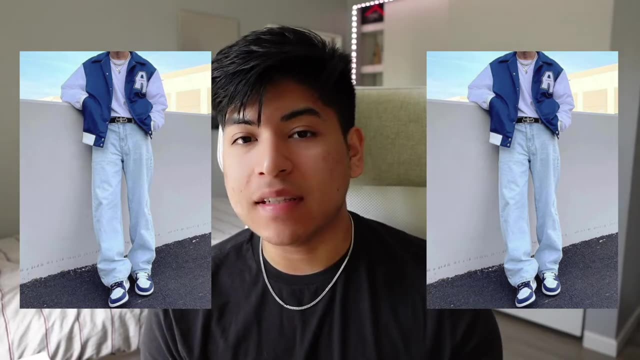 which just works very nicely And it just makes it look aesthetically pleasing. Same thing with the primary color on this one is green, but it incorporates different shades and tints of different pieces into the outfit, which gives it depth and layers to the outfit Next up we got analogous. 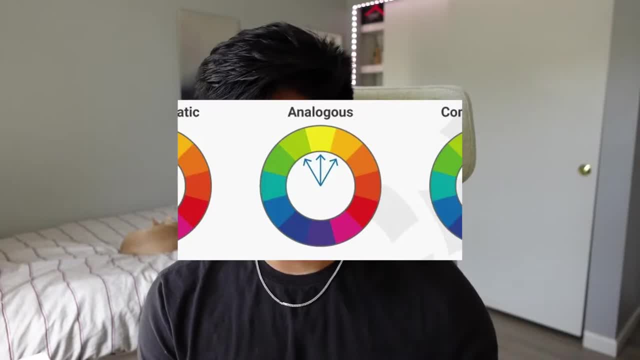 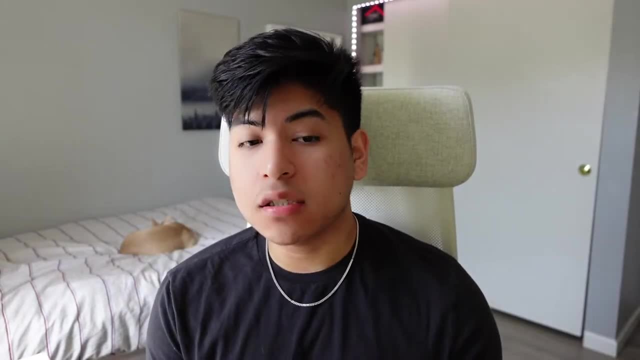 colors. Analogous colors are colors next to each other on the color wheel theory, Colors such as yellow and orange, orange and red, red and purple, purple and blue, so on and so forth. But analogous colors in fashion are mostly used to stay a part of a certain theme or aesthetic, such as like: 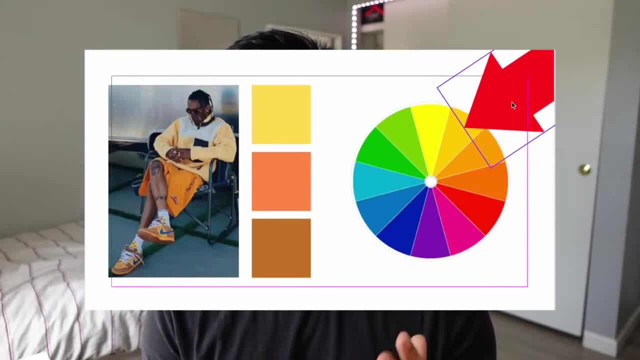 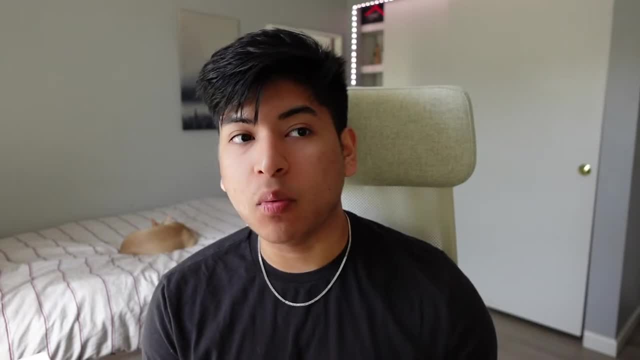 seasonal aesthetics, Like right now we're in summer, so you're probably going to see a lot to stay a part of that summer theme or, like fall, For example, you're going to see a lot more people wearing like beige, brown and black and also some orange, But analogous colors are really good to. 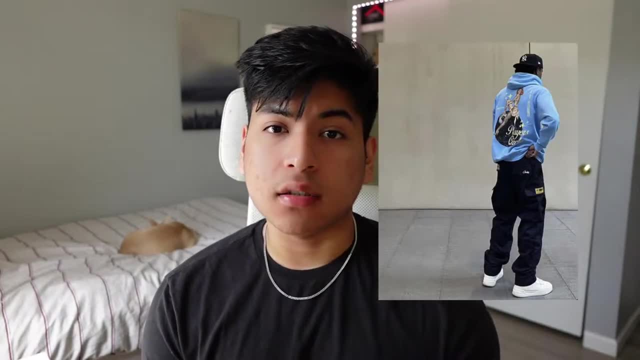 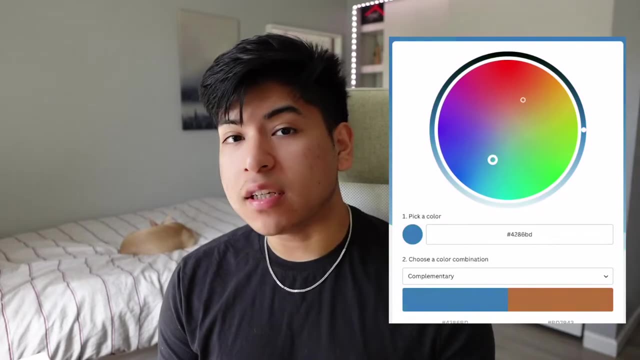 follow to stay a part of a certain theme or aesthetic, And they're also good for color blocking. Next up, we got complementary colors. Complementary colors are opposite sides of the color wheel, Colors such as yellow and purple, red and green, blue and orange, And these colors 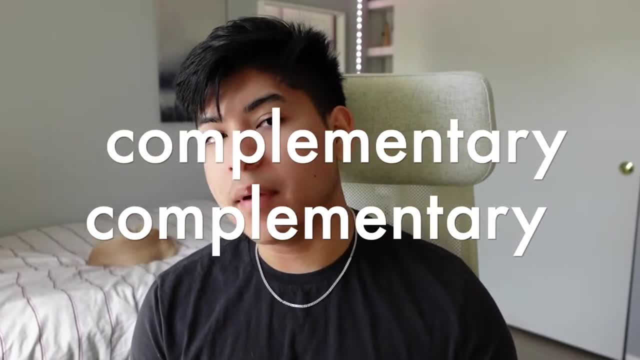 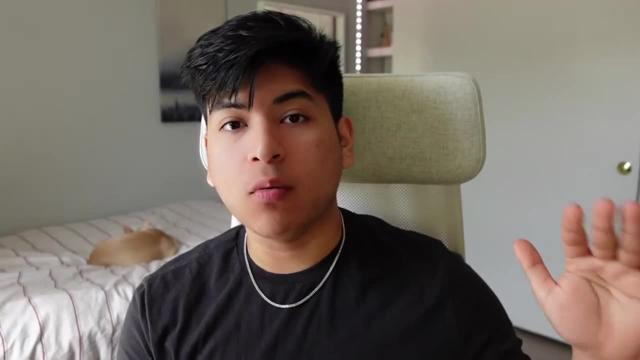 complement each other. They bounce off each other very well, hence the name complementary colors. And there's two ways to add complementary colors into your outfits. The first way is by splitting the top layer, incorporate one primary color and then, for the bottom layer, incorporate a. 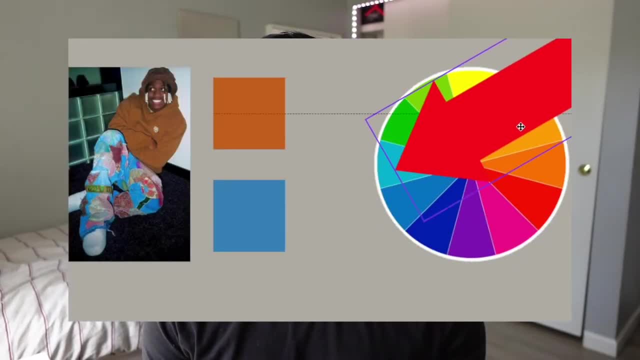 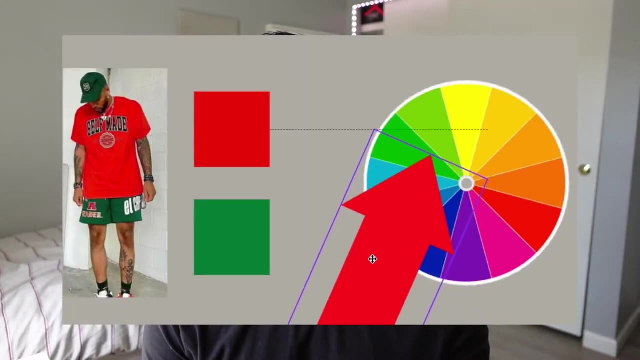 complementary color or vice versa, Like this one, for example: the top piece has an orange layer to it and the bottom is a blue layer, both of them being complementary colors and working well. And this one, too, has a red upper and a green bottom, both colors complementing each other, And this 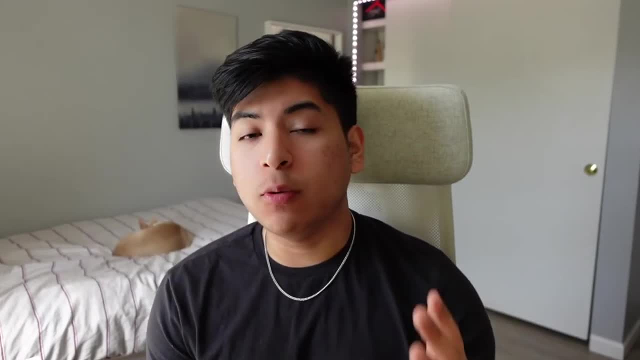 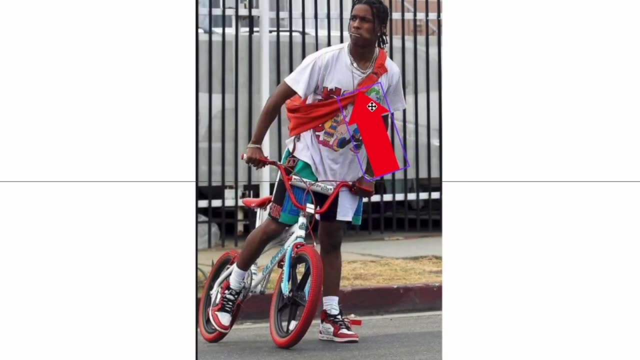 one too, purple and yellow working well together as well. And the second way to incorporate complementary colors into your outfit is by choosing two primary colors, such as this one- a white upper and a blue bottom, but incorporates a thin layer of a complementary color, As seen on. 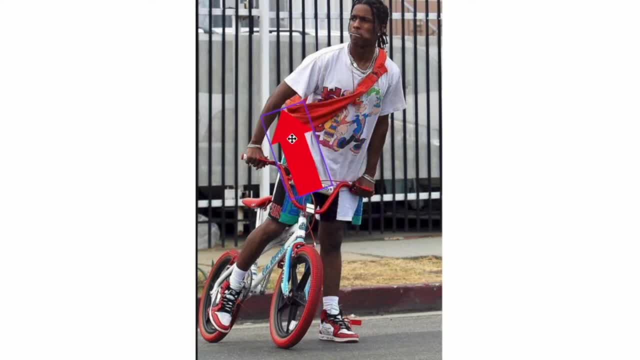 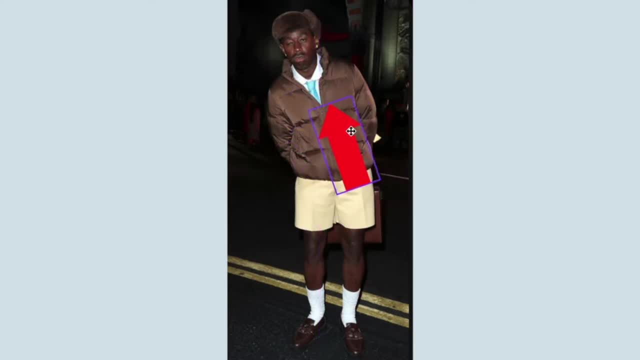 her and the shoes, pretty much incorporating subtle complementary colors into your outfits. Or like this one as well: a beige bottom and a brown upper, but he incorporates a thin layer of a complementary color of blue, Although it's not exactly opposite ends of the color wheel. 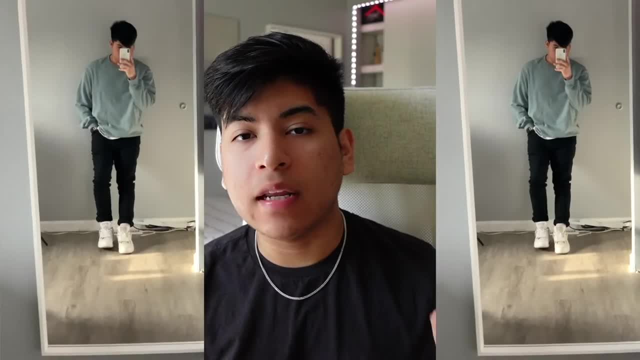 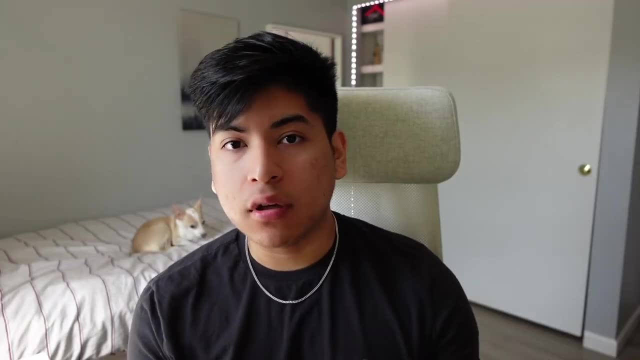 theory, it still works well. Or what I'm wearing right here? a light blue upper and a black bottom, but my pink socks match the saturation of my blue upper, which complements each other working well. Adding subtle complementary colors to your outfit just makes a big difference, and just